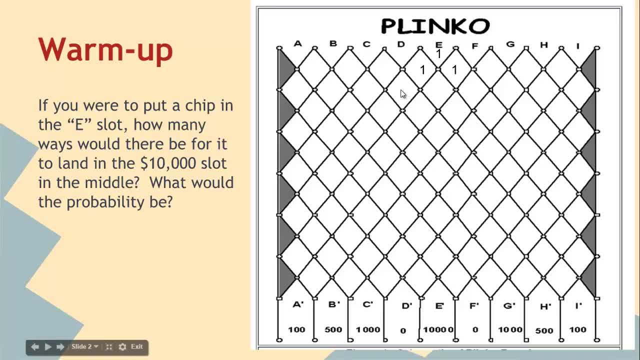 And so then there'd be one way for it to fall down. this way It would have to go straight, And so there's one way to go here, And there's actually two ways to get here. So you could hit this peg and then hit that peg and end up here, Or you could hit this peg and end up there. 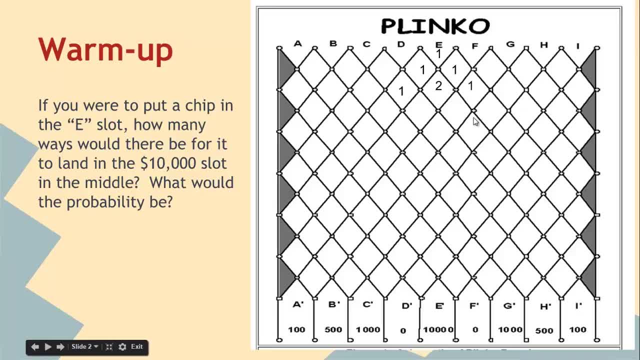 And then you could slide all the way down. For those of you guys that have seen this in 3U math, like you start to see what the pattern is that starts to develop, And it is Pascal's triangle. So you would have seen this in grade 11 university math. 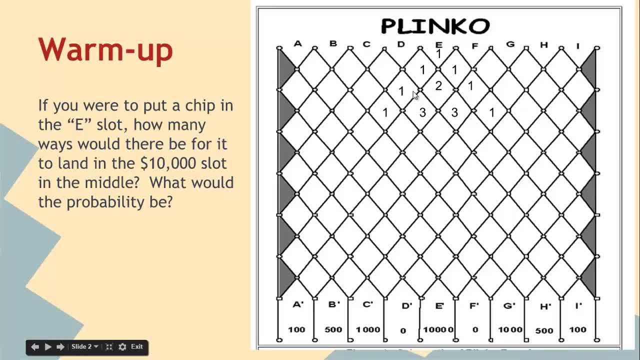 But if not, if you took 3M, then that's fine. But what we're saying is, if there's two ways to get here and there's one way to get here, that means that there must be three ways to get here, Like this is one way, And then there's another way here, And then a third way here, And so if we just add up these numbers that are above it, we get there, And so if we continue that way all the way down, you can kind of slow us down if you want to, or pause it. 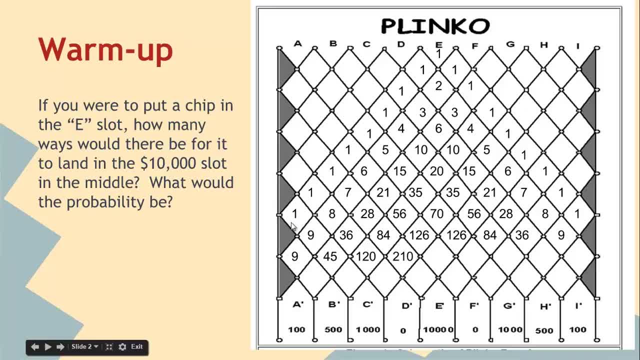 We see eventually- and here it's a little bit tricky, like because there's actually no left slot- It's just coming from the, it's coming from the top two here And here it's only coming from here. So there's nine, It's not like there's 10.. You don't add another one because you can't get here, But we keep going like that all the way down To get to the E slot. there's finally 924 ways- And the probability would actually be out of the total number of ways- to reach this bottom row. So it's 924 out of 434.. 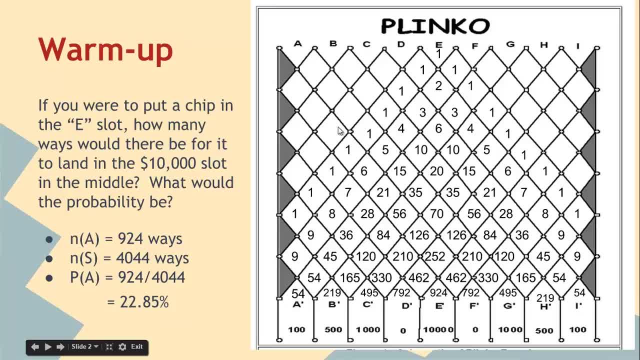 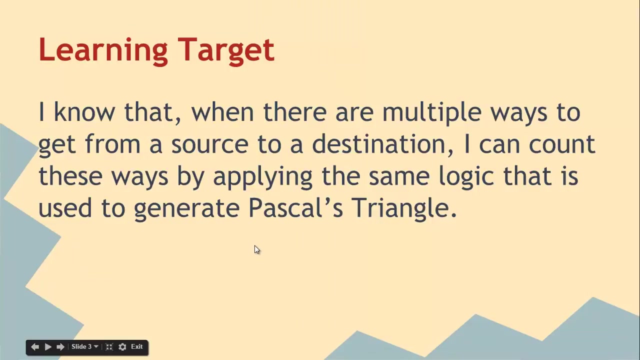 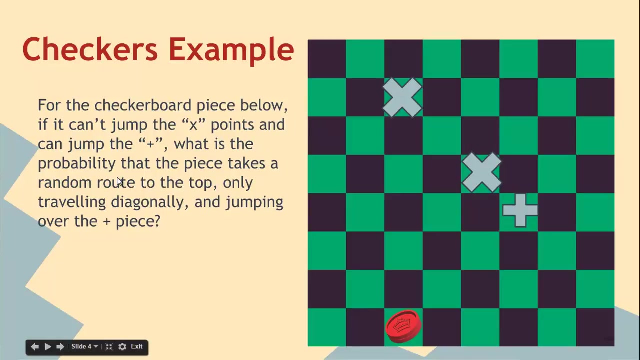 Which is about 23%. So I know that when there are multiple ways to get from a source to a destination, I can count these ways by applying the same logic that is used to generate Pascal's triangle. So let's see another example. Again, it's just kind of like a puzzle. It's more for games than for real life, But we will see a route question as well, or root question, or however you say it. 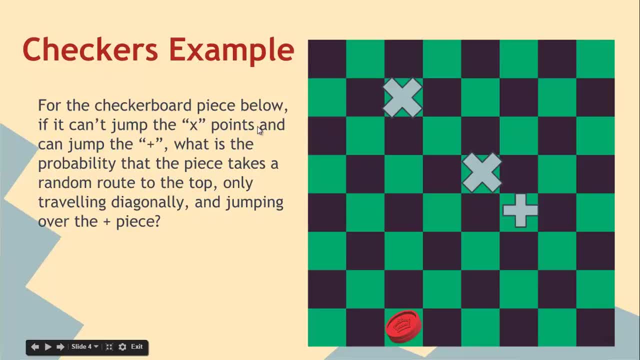 So the checker piece below, if it can't jump the X but it can jump the plus, what is the probability that the piece takes a random route to the top, only traveling diagonally and jumping over the plus piece? So the first thing you need to decide is how many ways to get to the top row and then how many ways go through that plus piece. 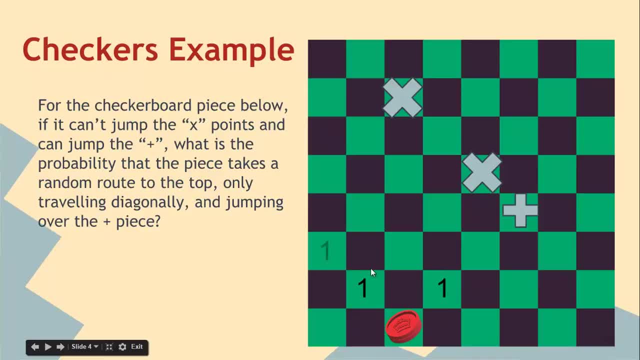 So there's one way to get here and one way to get there, One way to get here and two ways to get here. One, two, One way to get here, Three, Three, And we can't. We can't actually go there because there's somebody there, so we jump over it. 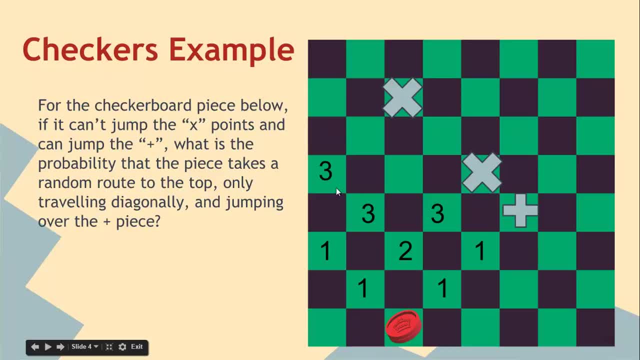 Three ways to get here because you're not coming from this side. There's almost zero here. So six ways to get here And zero ways to get there. It's helpful to actually put a zero there- And one way to get here because we can come from this side. 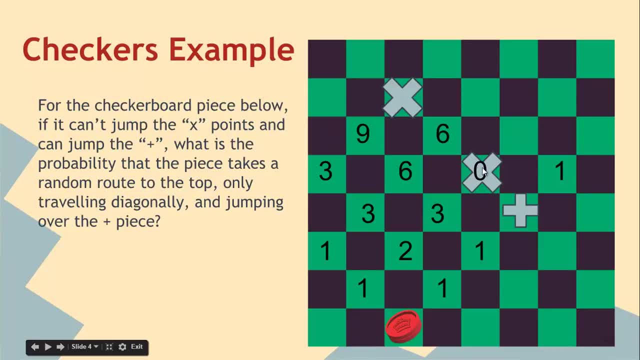 So nine here, six here. That's where the zero will help. It's just from there. And then one way here, because this is zero plus one, And one way here, because you can almost think of this as a zero too. 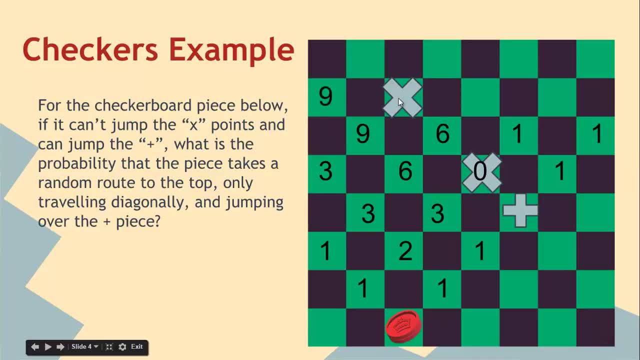 Nine ways to get here, Zero ways Seven. Two ways to get here, Nine ways to get here, Seven, nine and two. So if you add these ways up the random row there would be that number of cases. So there would be 27 ways to get to the top. 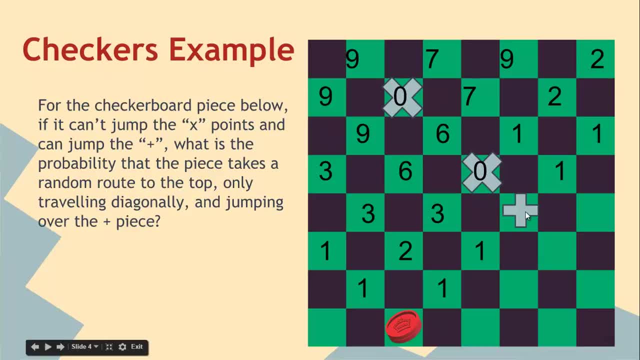 Now, if you actually had to go through that plus sign, what we do is we ignore all the rest. We can almost put zeros on the ones that have gone too far, but we can see that, like you have to go through this plus sign. 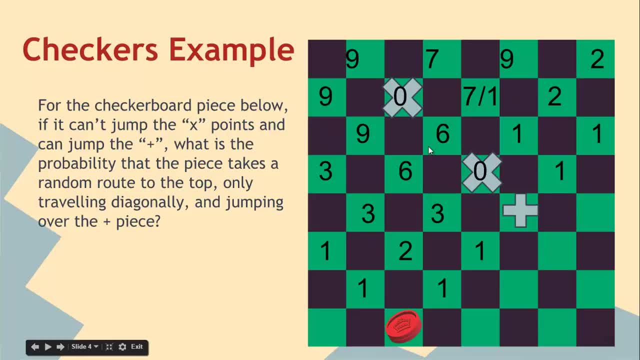 So there's actually only one way to get here now, because this would be not possible. There's zero ways to get here through the plus sign. You notice you can't go backwards. That means there's one way to get here and it's just through this one, because you can't come in from this side. 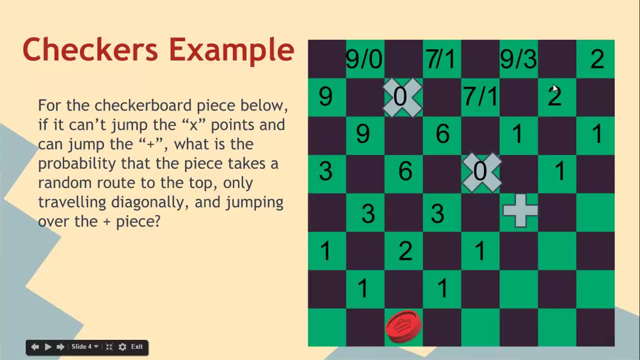 One plus two is three ways to get here. The two- all of the routes for the two have gone through the plus sign, so they're good- And then two here as well. So in total there are one plus three plus two, so the little dashes are the new numbers. 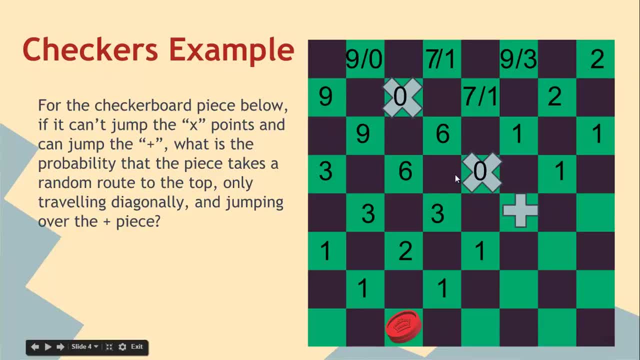 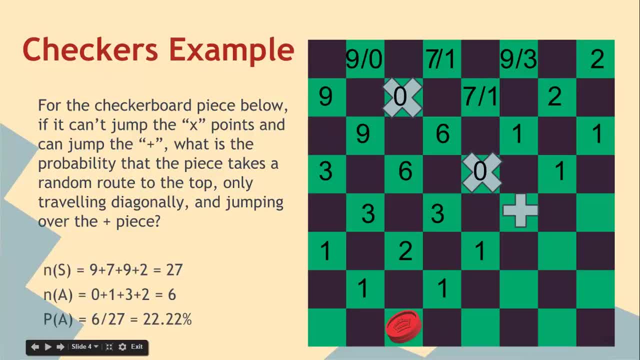 So n of s is the 27,, n of a is the zero, one, three and two, And so the probability of a is 22 percent. So the probability that you're going to go through the plus sign of a random route is 22 percent. 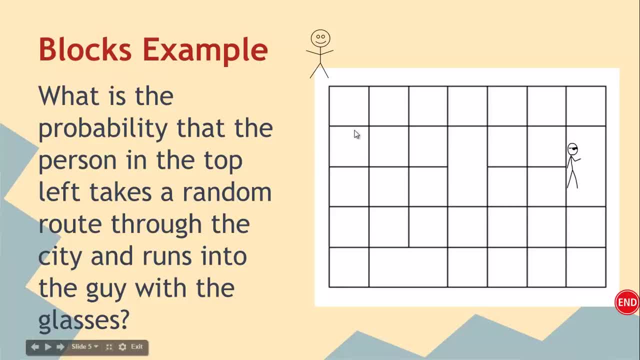 Block example. So this is where, like, you've got a city block and so some of the blocks may be doubled, So a building is here and you can't go through it. the building and here as well, and so you got to pay attention to where the lines are. but then 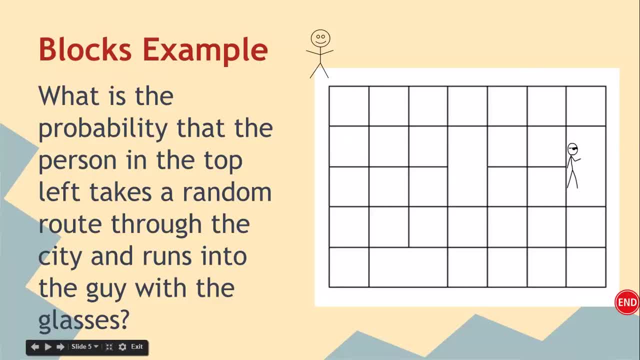 you've got like you can travel south and east, uh, to get to the end, but you can't go through the guy with the glasses, this suspected cool guy that maybe gives you a hard time. um, so we want to find out the the probability that we're taking a random route through the city and, uh, running into the guy. 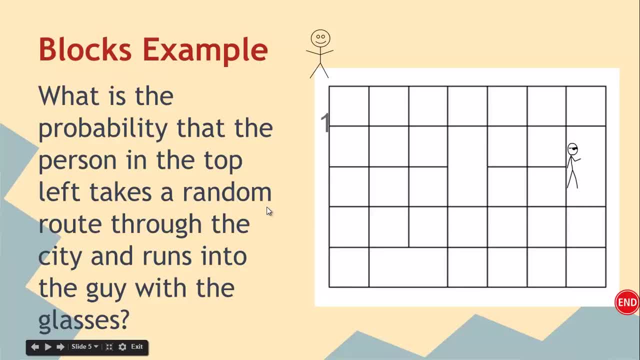 with the glasses, okay. and so again, we kind of draw those lines and so there's only one way all the way down here, because you, you're not going to go backwards. um, so you're going to be walking south and east and then pascal's triangle kind of picks up and there's no real change. 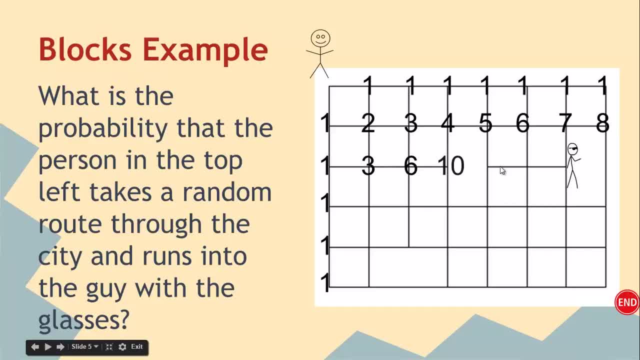 until we get to this point here where now we can't go through. okay, there's actually only five ways to get here, because we can't come from here. um, so that's where a lot of people will make a mistake, because they won't show what to do is the? 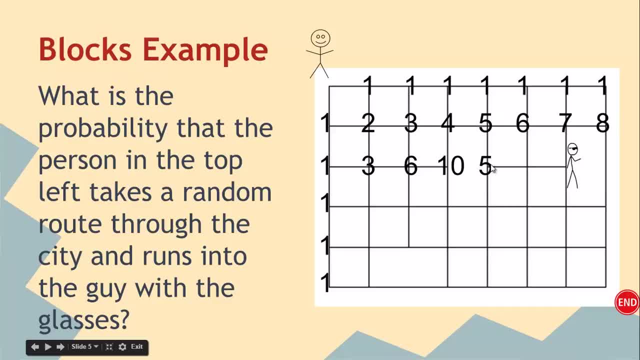 number just kind of carries down. it's almost like there's only five ways to get here. so there's the same five ways to get here. it's just one more dash. so you got 11 and 18, um. so we're trying to find out all the ways down to the end, not just through the guy with the glasses, uh, to do probability. so 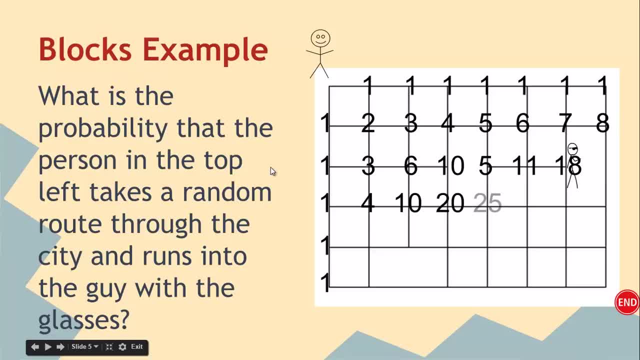 we've got to find out n of s first, and so then we can continue on with this, and we're going to start with our pascal's triangle. that this row is kind of normal. um, this row is kind of normal, just adding up then this one: um, again it's pretty normal too. it's just like 35 and 6. this 15 doesn't. 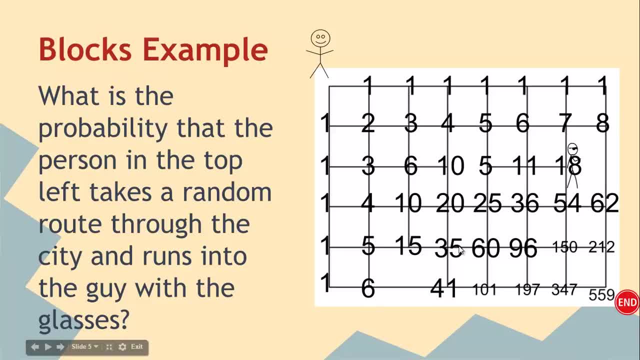 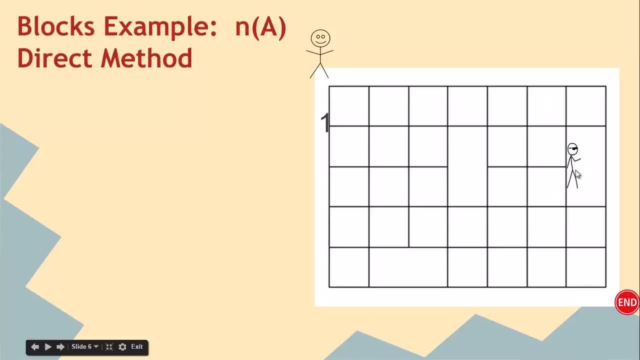 go anywhere, um, and so we end up with 559 roots to the end. so now, if we want to go through a guy with the glasses, what we do is we we do a direct way where we have to go through the classes and the guy with the glasses, and so we're going to just find out how many ways we can go there. 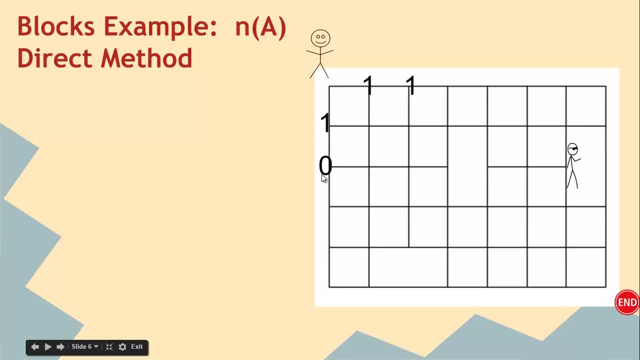 there's actually no ways here, because if we go through that way then we're already too far to get to the guy with the glasses. we'd have to go down here and back up, so we put a zero there and there's actually zeros all the way down and here as well, because if we go that way then we've 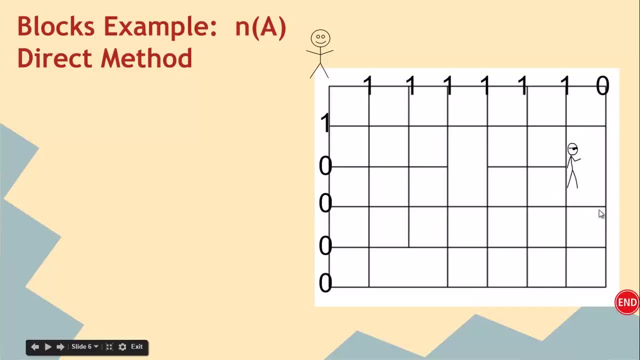 gone too far and we can't go through the guy with the glasses unless we backtrack. so we put a zero. um, put a zero here, although there should be seven ways, because again we don't want to. we want to go through the guy with the glasses. put a zero there because we would have gone too far. so there's two. 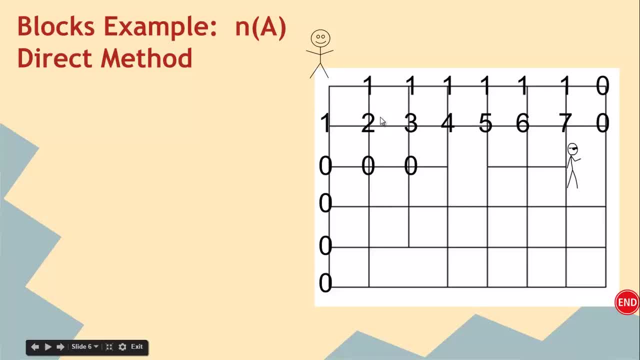 ways here, but then there's no ways without with going through the guy. uh, we can still go there and still meet him, but we can't go down anymore. so 11 and 18, um, we can't go here. there's only really this way. here is 18 and then 18 again. so there's 18 and there's 36 ways, because if we